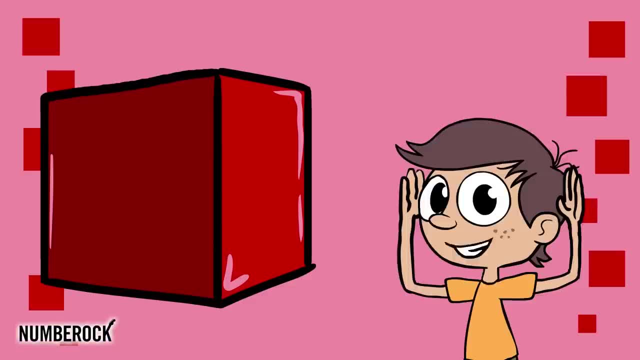 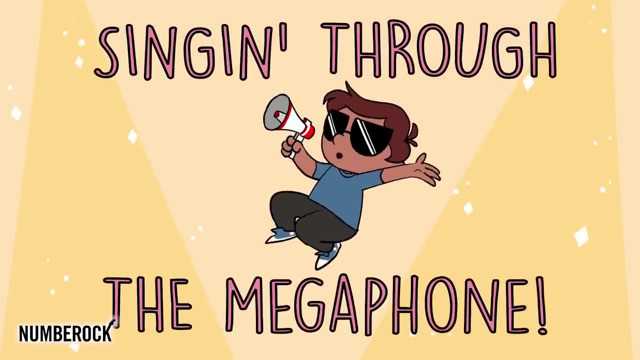 Let's go. Spear Cylinder- Pyramid- Cube Cone Singing through the microphone. Spear Cylinder- Pyramid Cube Cone Singing through the microphone. Spear Cylinder- Pyramid Cube Cone. All 3D shapes. 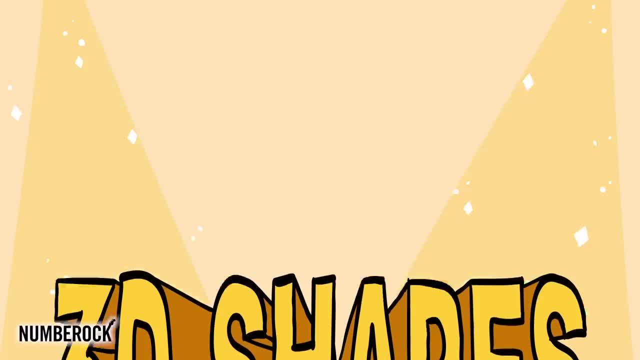 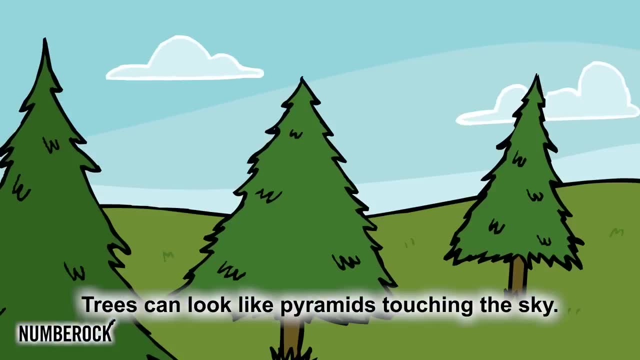 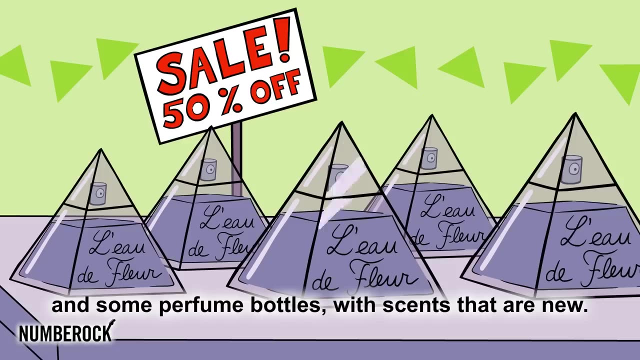 3D shapes. The Egyptian pyramids stand very tall. Closed umbrellas look like pyramids before rainfall Trees can look like pyramids touching the sky- A pyramid block of cheese. give it a try. Some house rooftops are pyramid zoo And some perfume bottles with scents that are new. 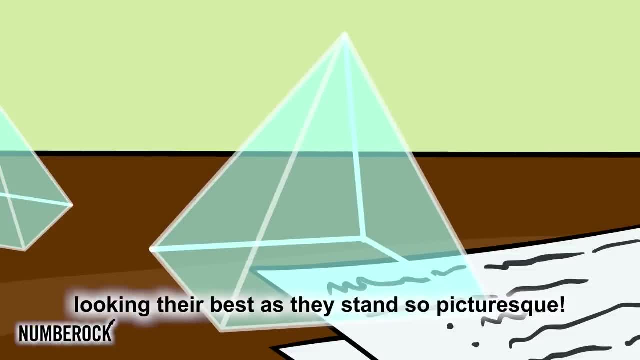 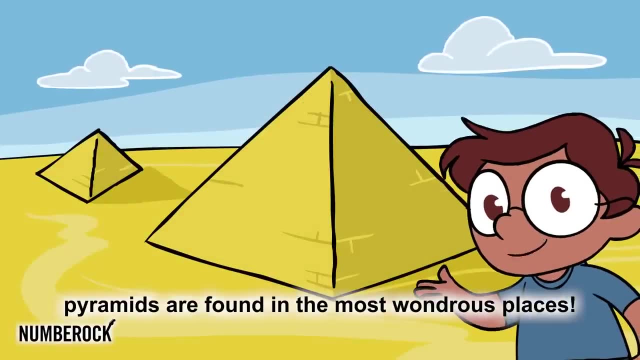 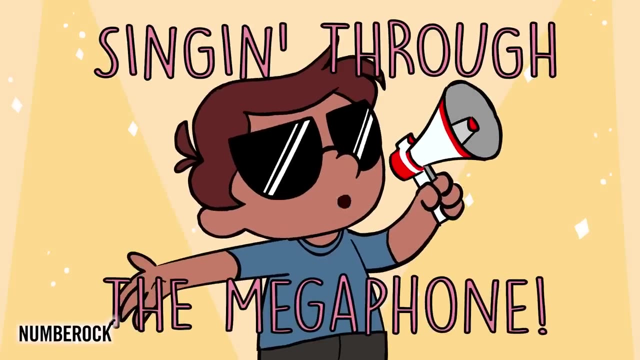 Pyramids shape paperweights on a desk. Look in their best ass. they stand so picturesque With a base and apex and faces. Pyramids are found in the most wondrous places. Let's go: Spear Cylinder, Pyramid, Cube Cone Singing through the microphone. 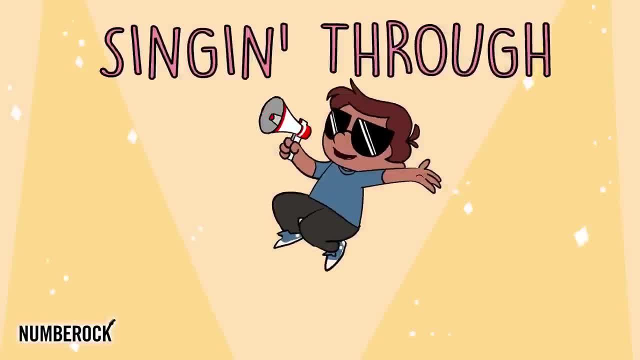 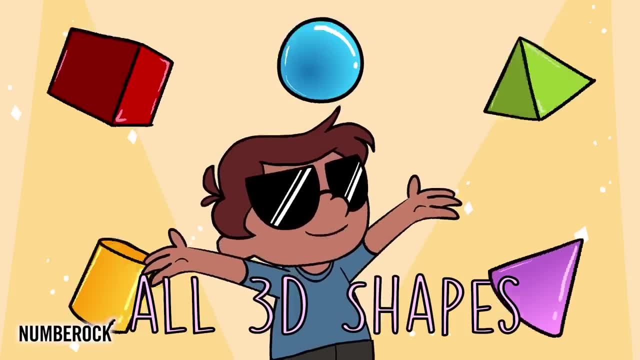 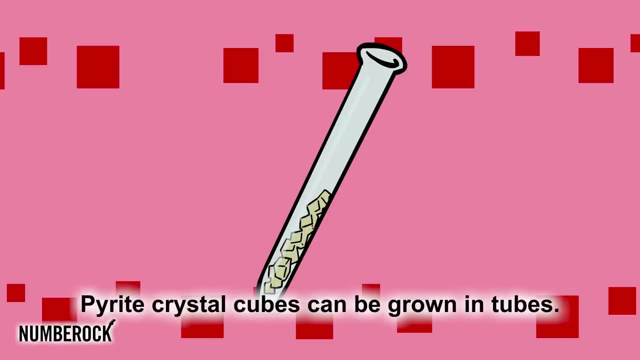 Spear Cylinder, Pyramid Cube Cone Singing through the microphone. Spear Cylinder, Pyramid Cube Cone, All 3D shapes. 3D shapes: If you've rolled dice, then you've rolled cubes. Iron crystal cubes can be grown in tubes. 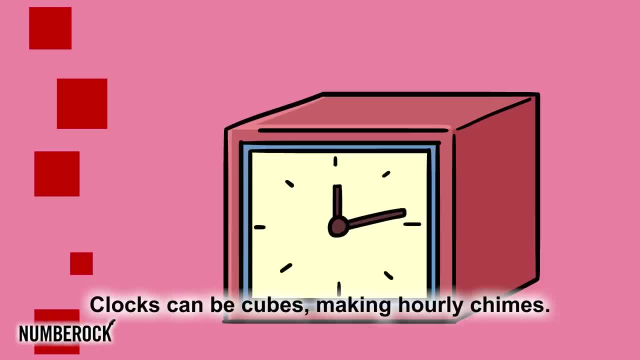 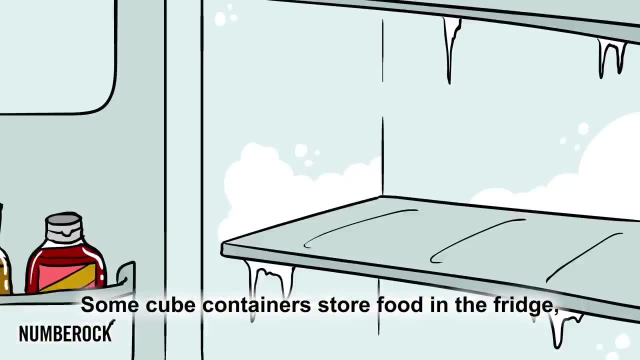 Blocks are cubes much of the time. Clocks can be cubes, making hourly chimes. A box in the mail might be a cube shape. Ice cubes can cool your ice cream shake. Some cube containers store food in the fridge And some concrete cubes can hold up a bridge. 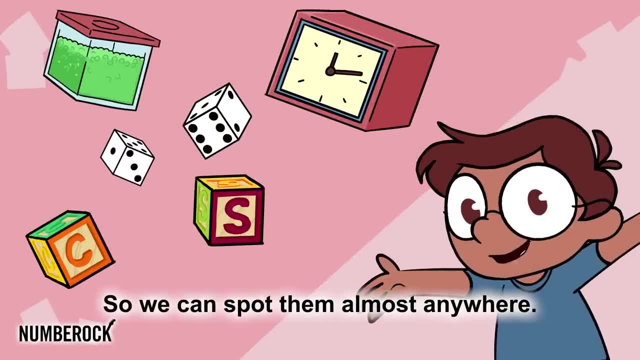 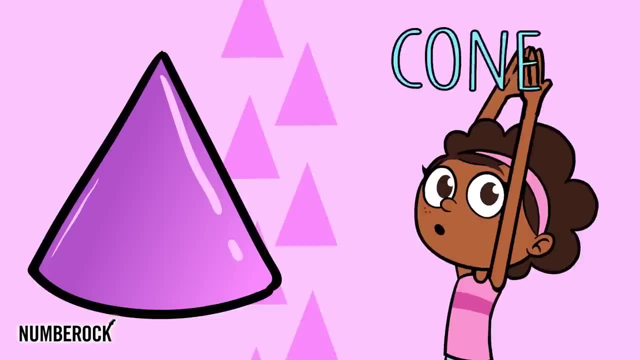 The faces of a cube are all a square, so we can spot them almost anywhere. Let's go. Spear Cylinder Pyramid Cube Cone Singing through the microphone. Spear Cylinder Pyramid Cube Cone Singing through the microphone. 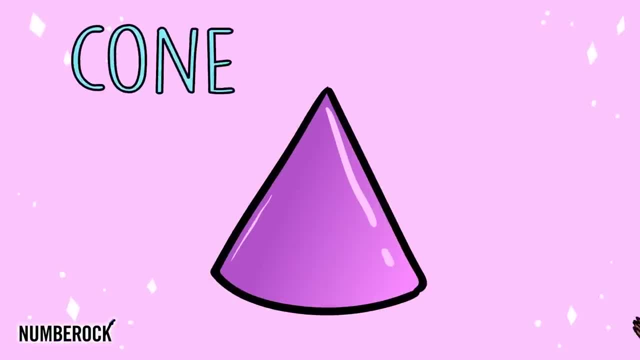 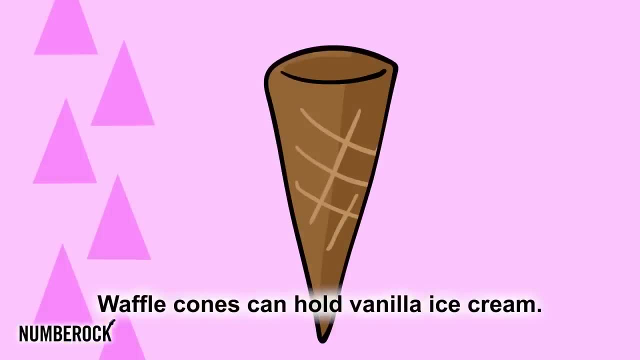 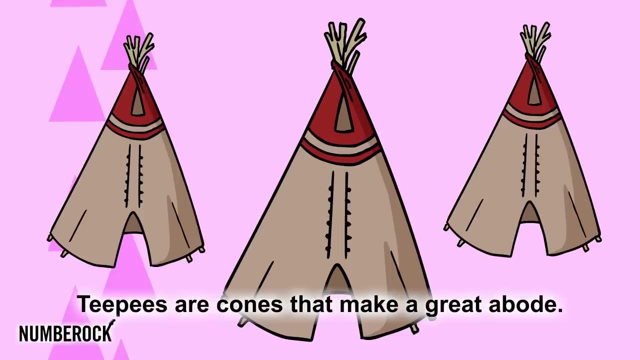 Spear, Cylinder, Pyramid, Cube Cone, All 3D shapes. 3D shapes. Waffle cones can hold vanilla ice cream. Hats on witches are cones that might make you scream. Orange cones can show dangers in the road. Teepees are cones that make a girl scream. 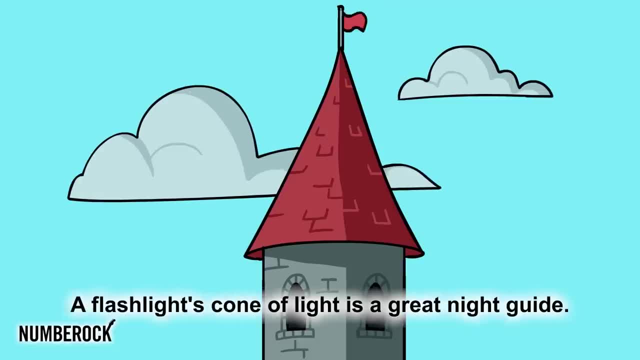 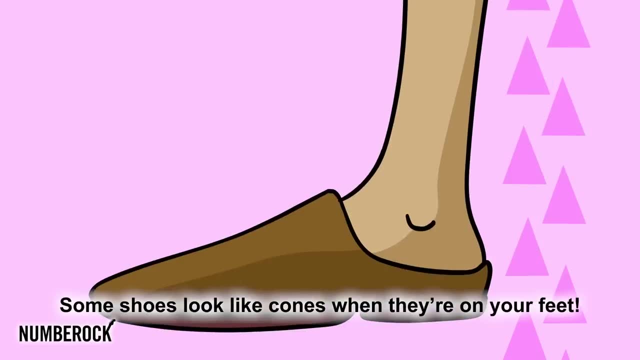 A great oboe Castle. turrets are cones to watch outside. A flashlight's cone of light is a great night guide. Cone-shaped cups may hold something to eat. Some shoes look like cones when they're on your feet, With a circular base and a pointy vertex. cones are always a favorite 3D object.